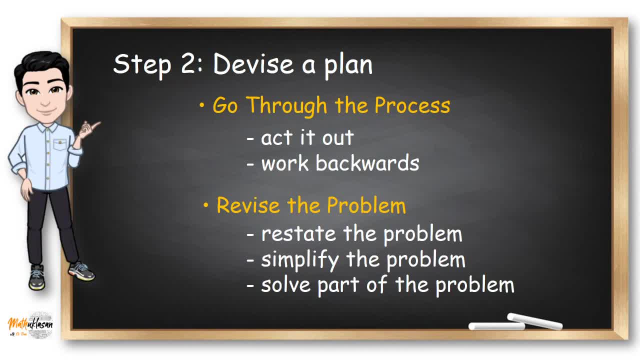 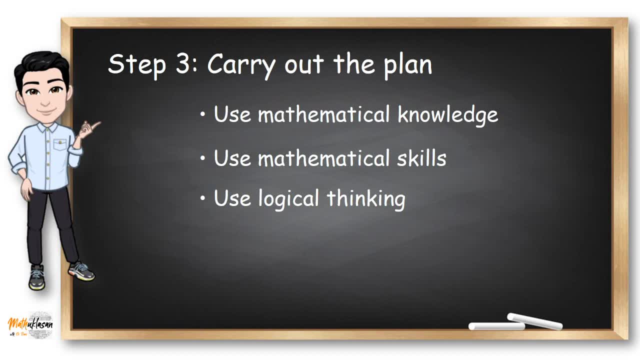 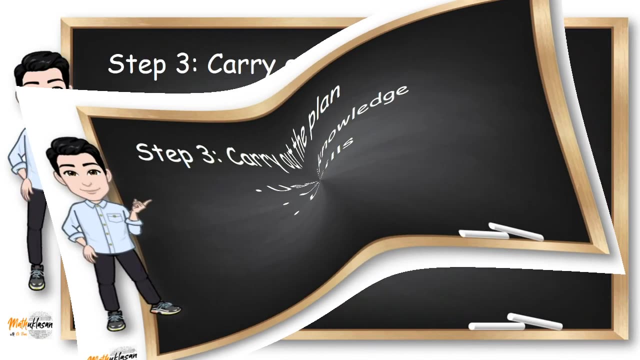 in the video. now, if you have a solid strategy or plan for the solution, we can carry out this plan by using our mathematical knowledge skills and logical thinking. this is the solution part in the problem solving process. after finding a correct solution or answer for the problem, we need to. 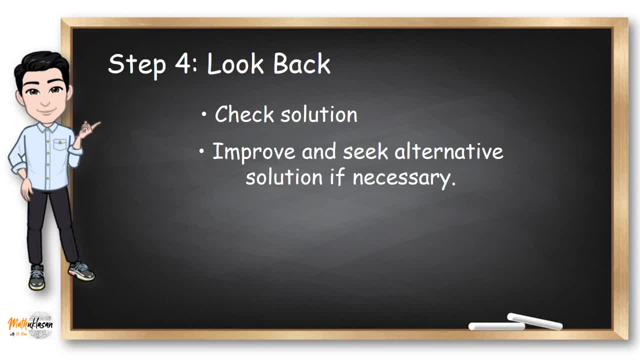 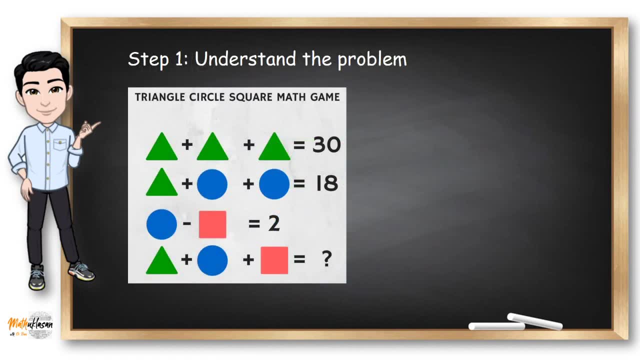 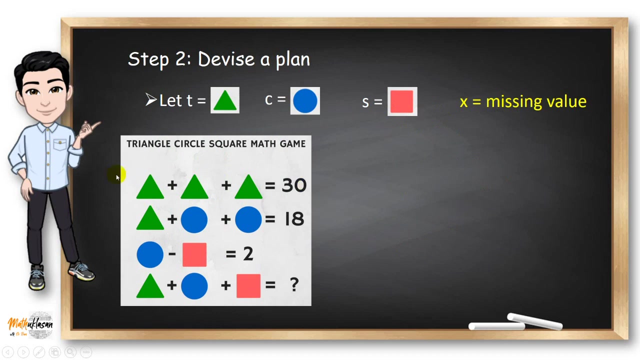 check the solution for us to improve and seek alternative solutions if necessary. for example, by looking at the problem, we can see that shapes represent numbers and the first three equations are clues to find the missing number in the last equation. whenever i see such problem in facebook, i always translate these figures into variables. 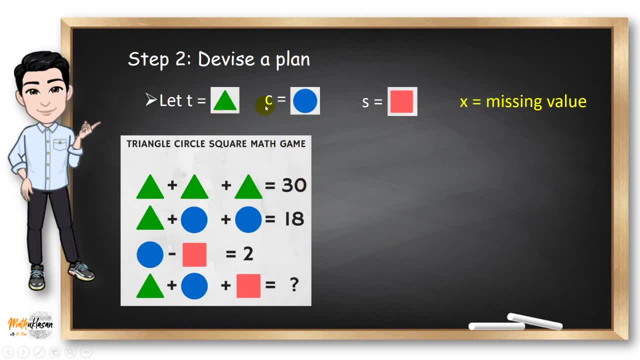 so in this case i let t be. the triangle c represents or represents the circle s for the square and x for the missing value. by rewriting the first equation, i will change these triangles into letter t, so i'll have t plus t plus t equals 30.. for the 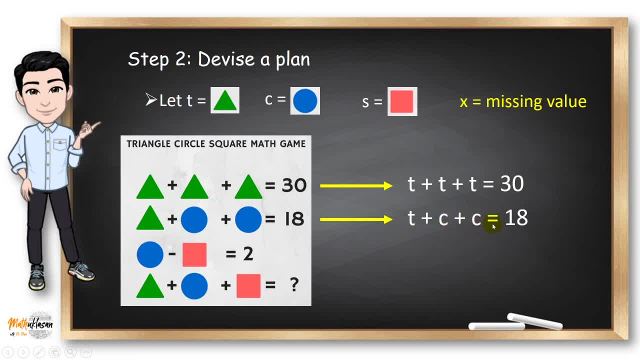 second equation, i'll have t plus 2c's equals 18.. for this third equation, i'll have c minus s equals 2, and for the last one, i will have t plus c plus s equals x. now, by using my knowledge in algebra, i 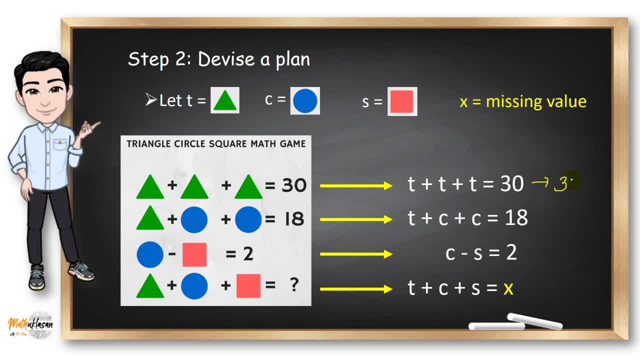 know that i can rewrite the first equation into just three things. so right now let's look what happens. if you add t and 2c as an einzige formula, the expression will work just like this. so here we are being given a solution for the third formula. 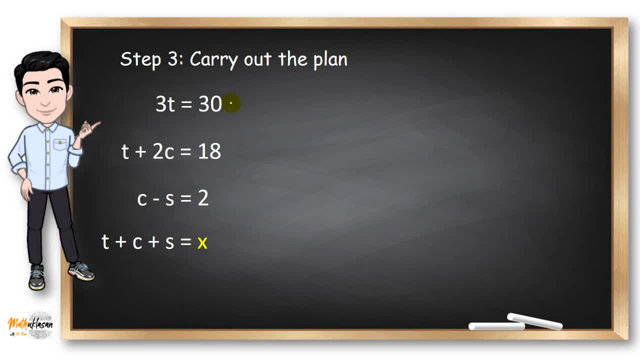 now, from here i proceed to break this Minecraft非常 glass box into smallerlings For T. in the first equation we need to divide both sides by 3 so that T is just equal to 10, because 30 divided by 3 is 10.. 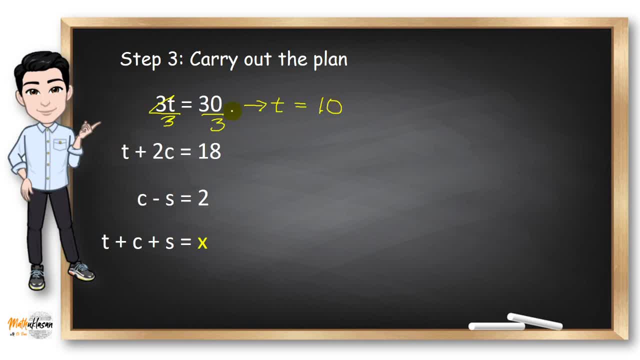 Now, if you don't have a knowledge in algebra, you can just think of a number that you need to multiply to 3 for us to have 30, and that is 10, right Now, since we all know that T here is 10,, we can now solve for the remaining value of C. 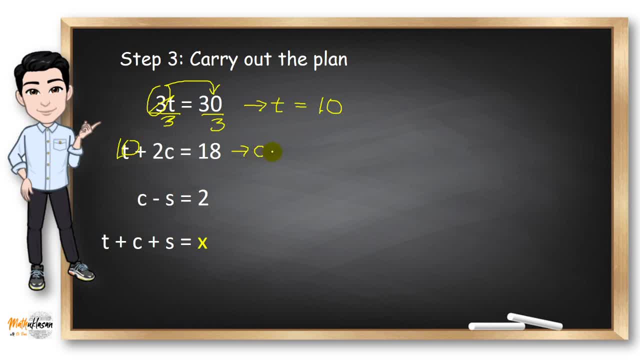 By using your knowledge again, in algebra, C will be equal to 4.. Or you just think of a number that you need to multiply to 2, and multiplying it to 10 will give you 18.. That is, C equals 4.. Now, since C here is equal to 4.. 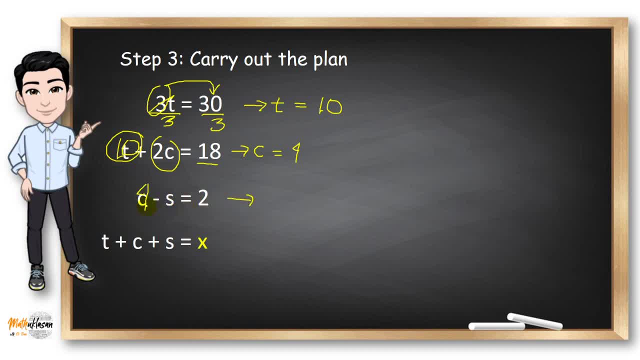 We just need to think of a number that we need to subtract from 4 for us to have an answer of 2.. So S must be 2, right? So since we got the values of T, C and S, we can now rewrite this equation into: 10 plus 4 plus 2 equals X. 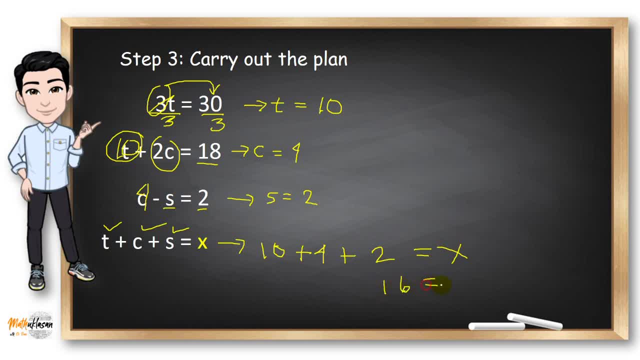 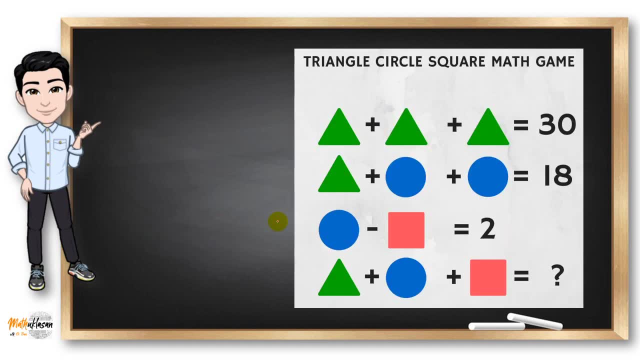 So that our final answer for X is 16. 16. Yep, that's it, But we don't stop it there, guys, because we need to look back and check our answer. We have found out that T is equal to 10.. 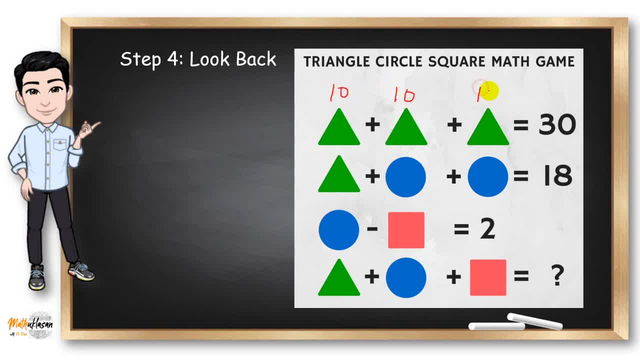 So if this triangle is 10, adding 3 tens will give us 30. So it's correct on the first equation. We know that or we have found out that triangle is 10 and the circle is 4. So adding 10.. 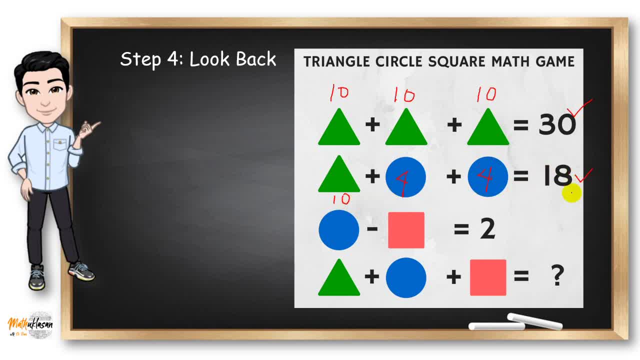 10 and 2 fours will give us 18.. So it's also correct. on the second equation: If the circle is 4 and the square is 2, then 4 minus 2 is equal to 2.. That is definitely correct. 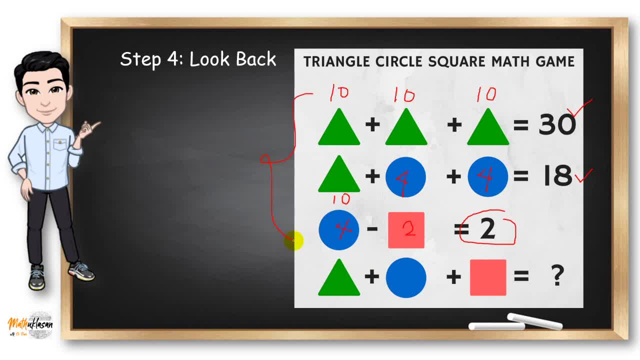 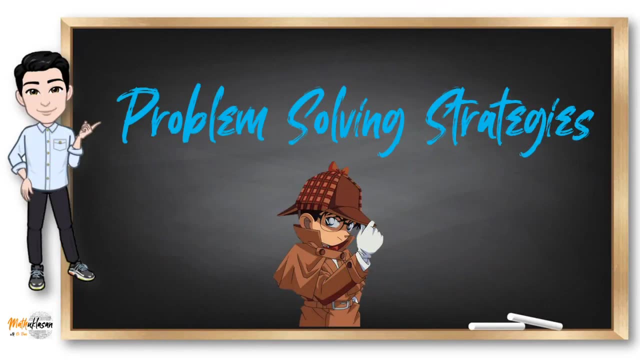 And by claiming or by confirming that these three equations are correct, we can now say that this is really 10,, this is 4, and this is 2. So that our answer is really 10. 16.. Aside from solving a lot of problems, the best way to become a skilled problem solver is to learn many strategies. 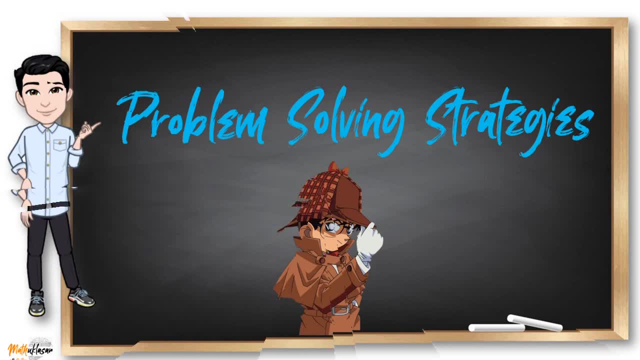 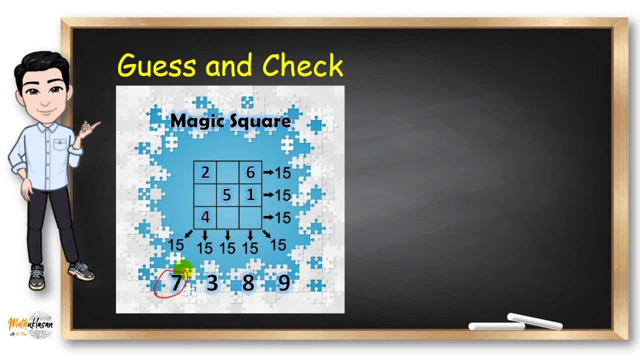 And here are some of the useful problem solving strategies. By looking at this magic square problem, we can see here that we need to distribute these four numbers in the cells So that the sum of, let's say, this diagonal pattern, The diagonal pattern, will give us 15.. 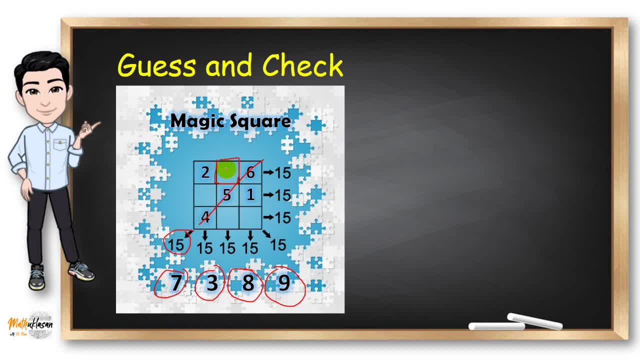 And also, if we are trying to put a number here in this cell, the sum should also be 15.. And for this I'm planning to use the guess and check strategy, because we need to think of an answer that might work, and then we need to check our guess. 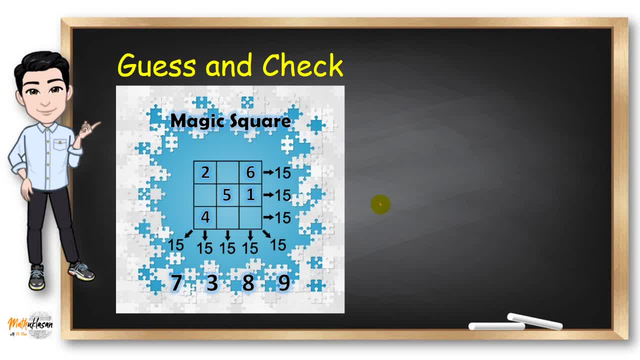 So in this case you can pause the video if you want to answer it first on your own and then continue the video to see the final. So let's start writing our guesses so we can start seeing patterns. So this is 2 and 6.. 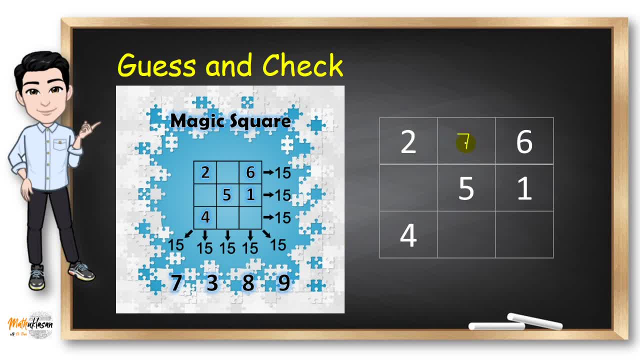 2 plus 6 is 8.. So this must be 7, because 7 plus 8 is 15.. How about this cell? 5 plus 1 is 6.. So this must be 9, because 9 plus 5 plus 1 is equal to 15.. 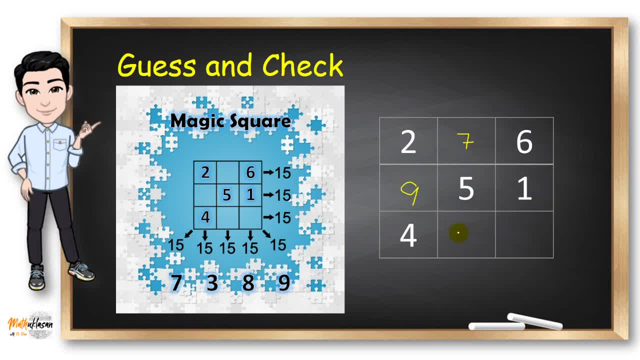 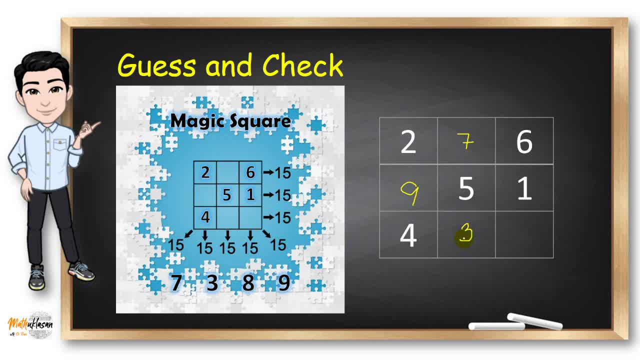 So this must be 3 for it to become 15.. Now I just need to add 6 plus 1 equals what 8 for it to become 15.. But remember that we need to look back, So we need to check our answers. 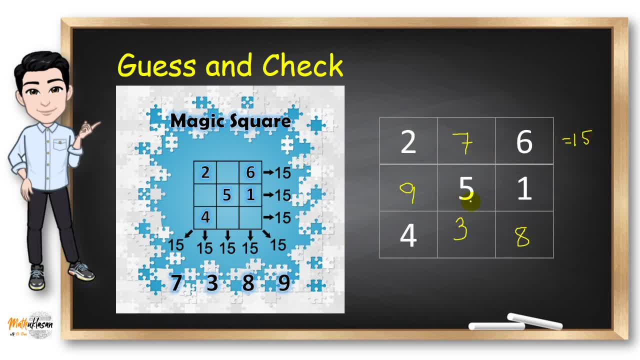 2 plus 7 plus 6 is 15.. So 9 plus 5 plus 1 is also 15.. 4 plus 3 plus 8 is also 15.. How about the sum on the vertical patterns? 2 plus 9 plus 4 is 15.. 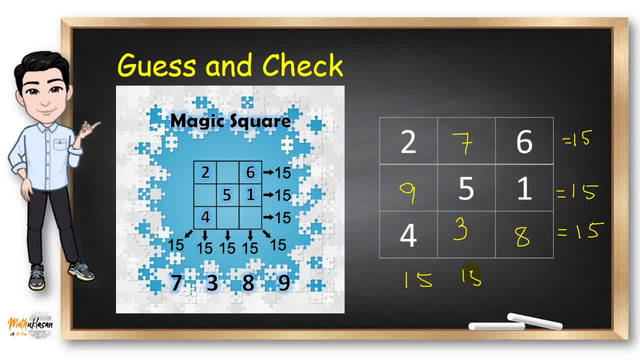 7 plus 5 plus 3 is also 15.. 6 plus 1 plus 8 is also 15.. How about this diagonal? Yes, 2 plus 5 plus 8 is still 15.. So by doing this repeatedly, 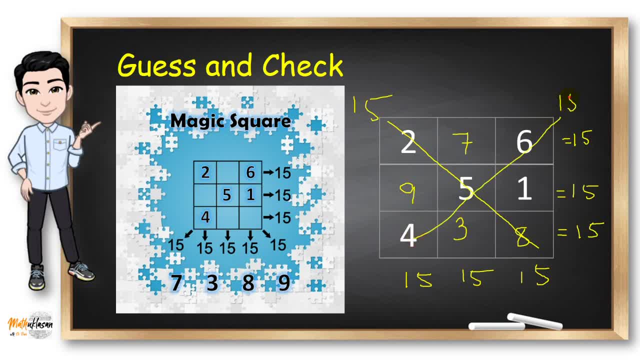 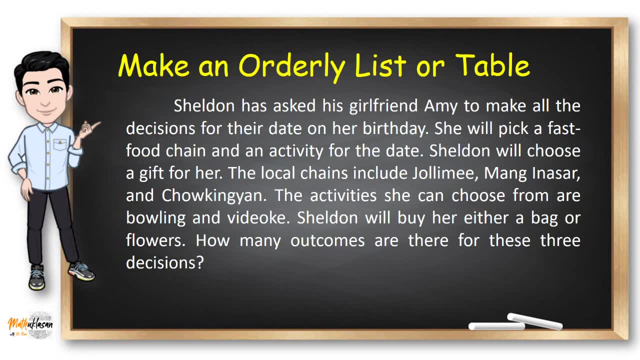 we can confirm now that our answer is correct. Making a list or a table is a way to organize data presented in a problem. This problem-solving strategy allows us to discover relationships and patterns among data. In this problem, Sheldon has asked his girlfriend Amy to make all the decisions for their date on her birthday. 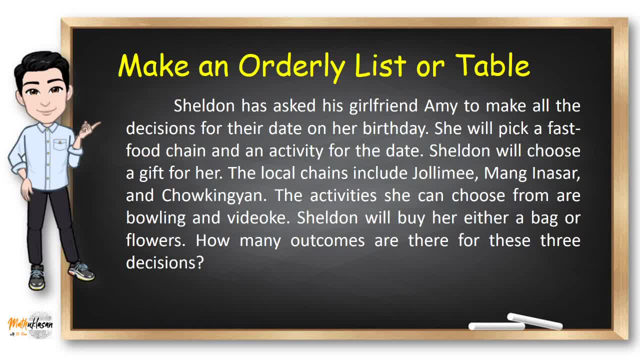 She will pick a fast food chain and an activity for the date. Sheldon will choose a gift for her: The local chain. The local chains include Jollibee, Mang, Inasar and Chowking Yan. The activities she can choose from are bowling and video games. 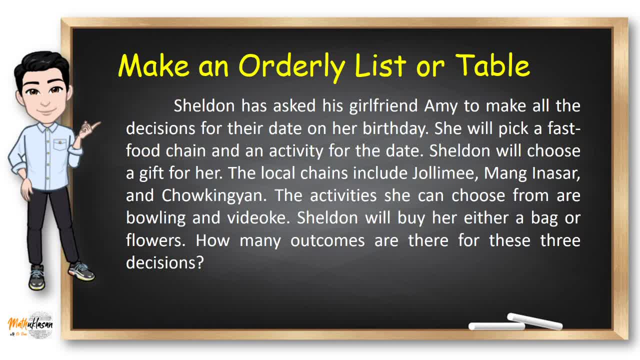 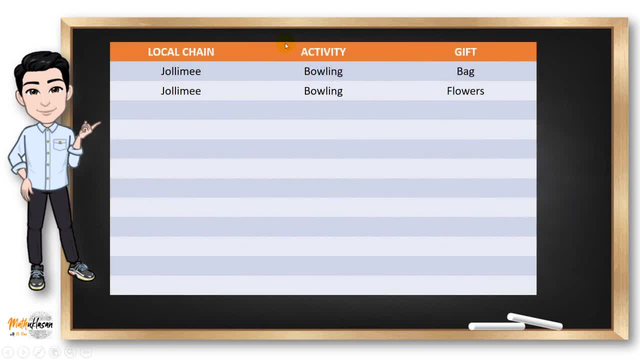 Sheldon will buy her either a bag or flowers. How many outcomes are there for these three decisions? We start our list with Amy choosing Jollibee and bowling for the activity, But Sheldon will either choose bag or flowers for the gift. So we have two outcomes right away. 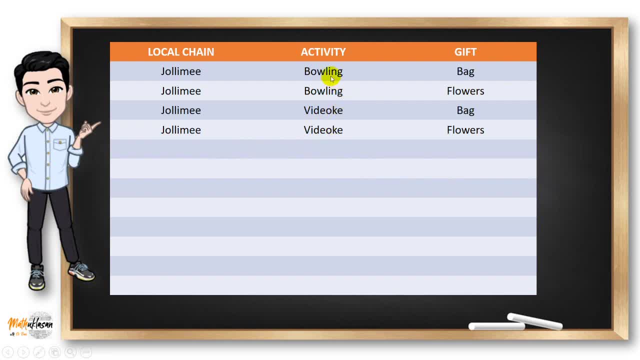 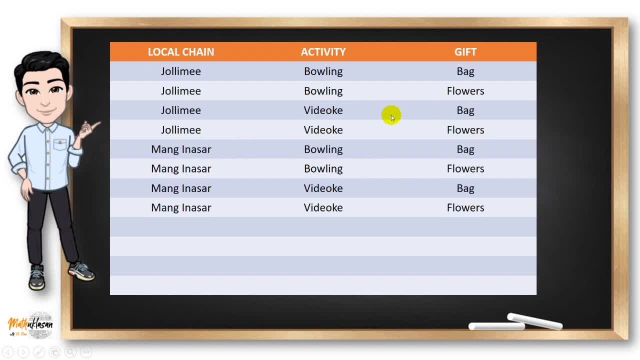 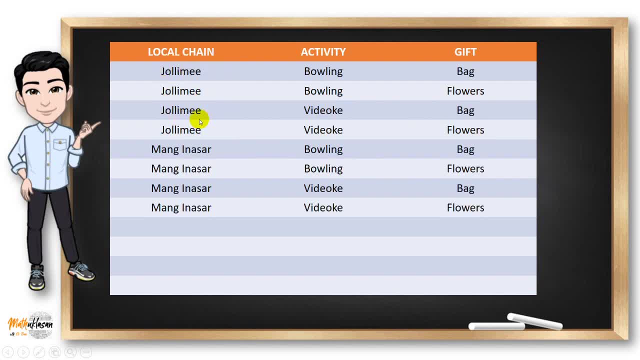 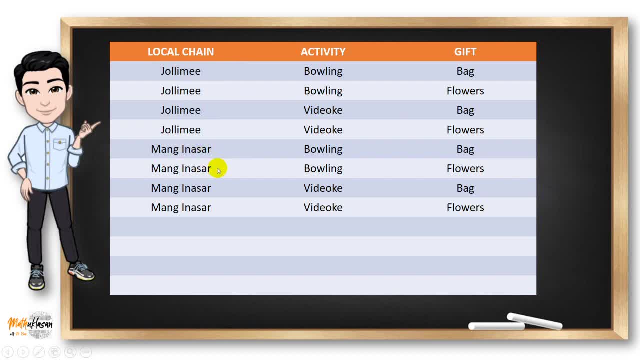 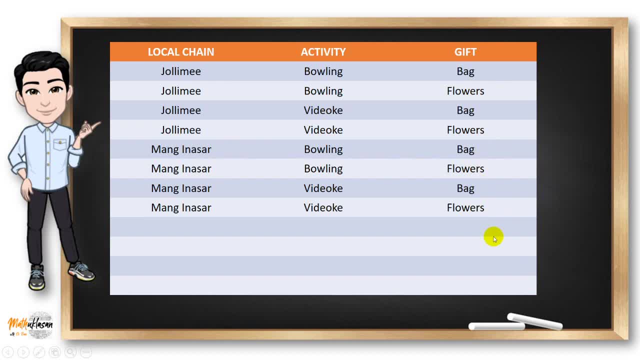 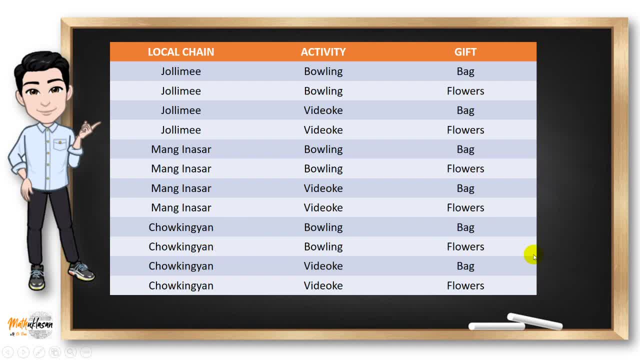 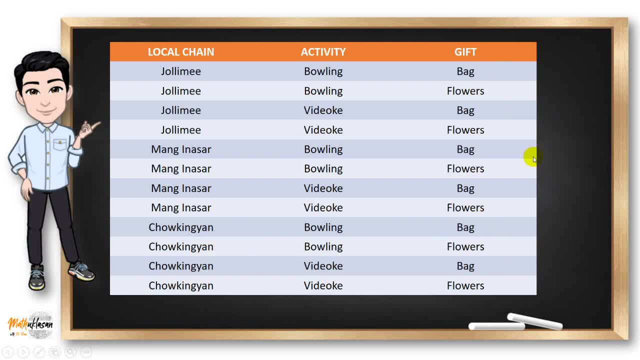 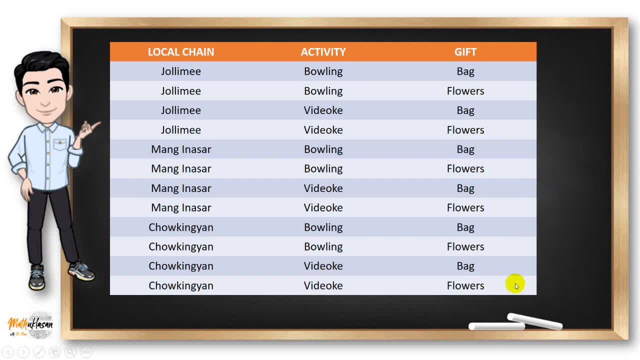 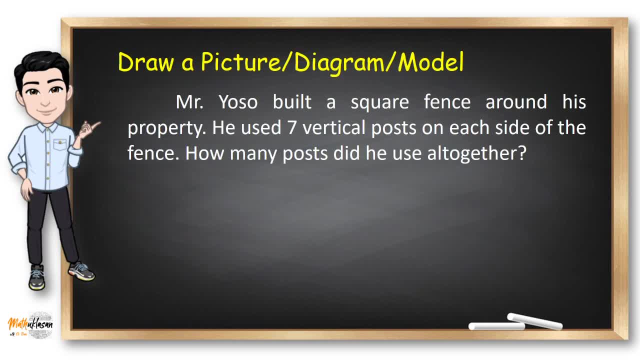 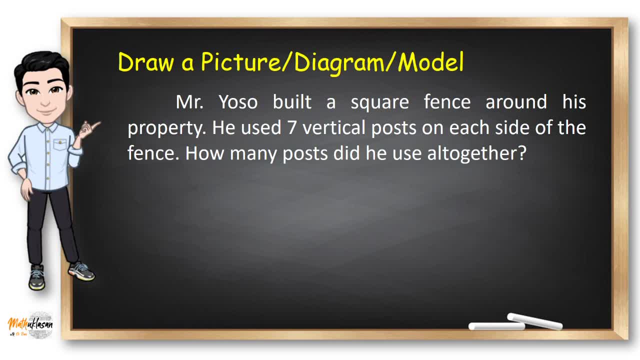 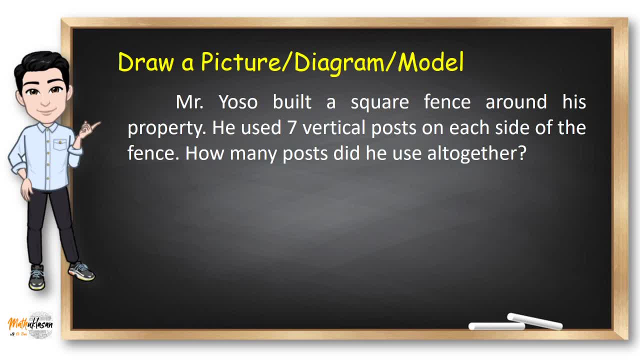 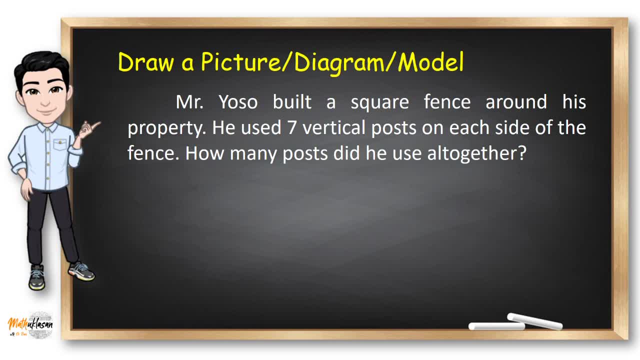 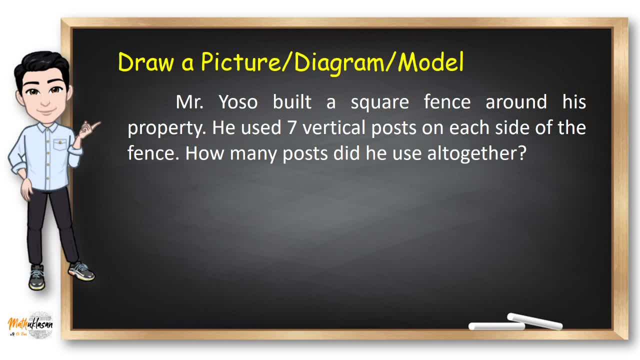 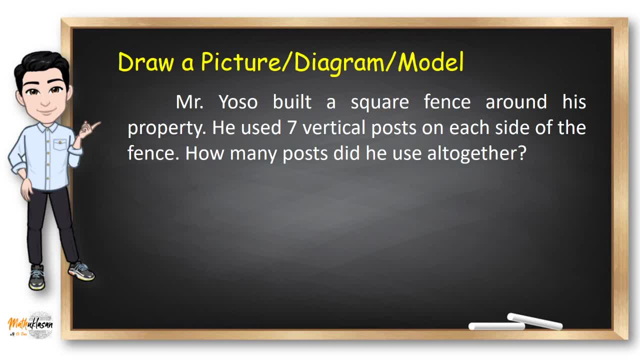 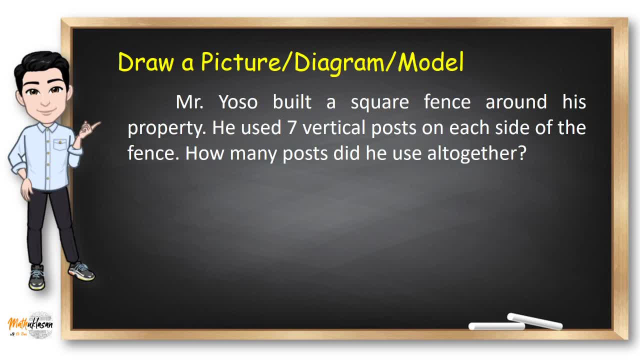 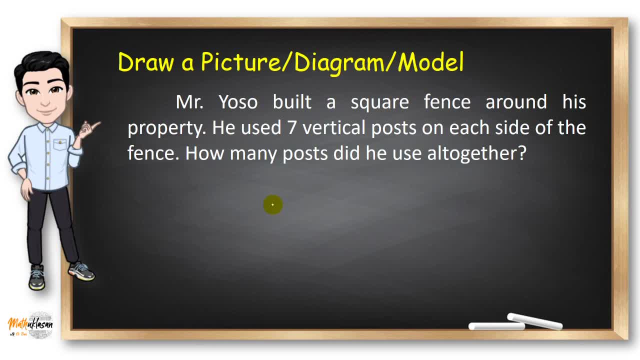 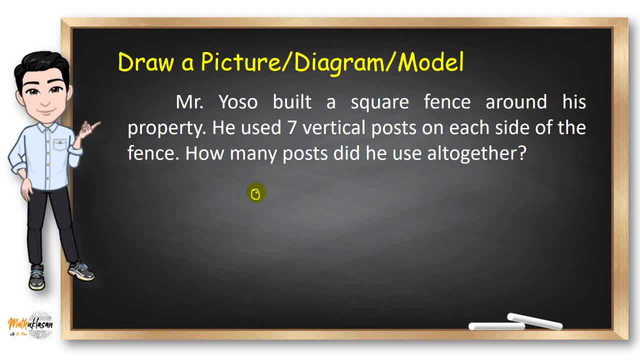 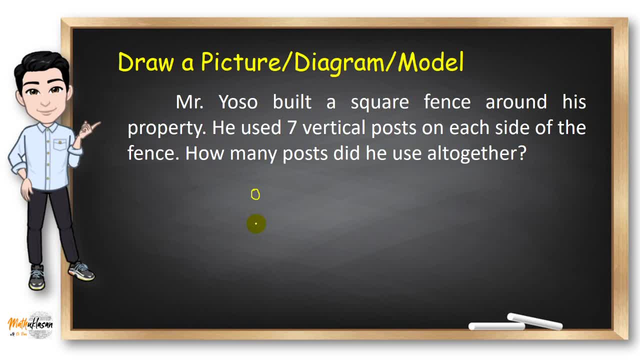 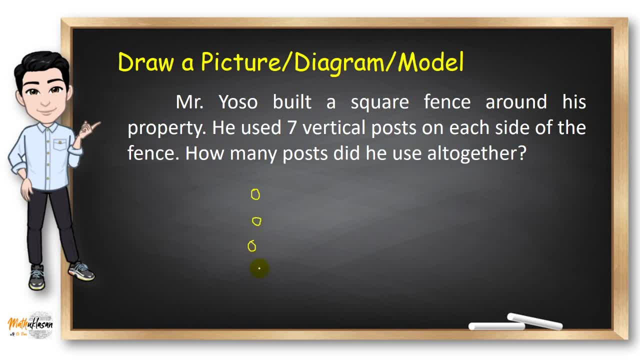 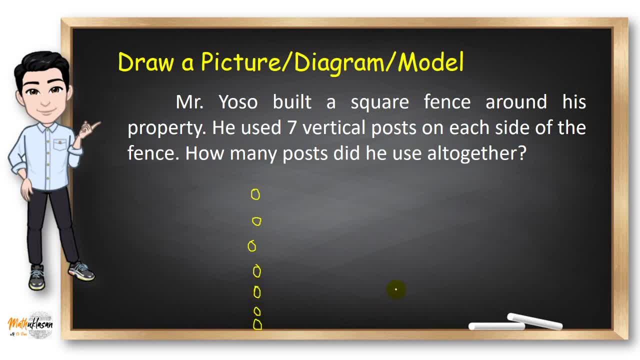 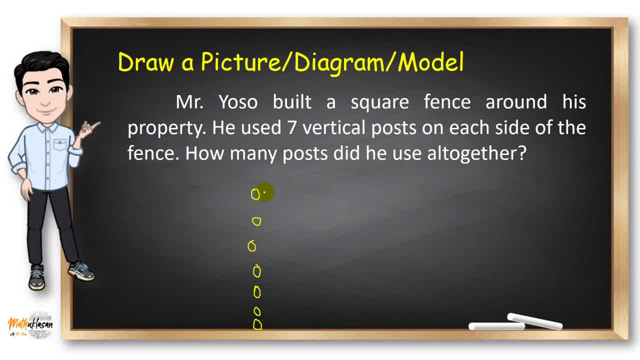 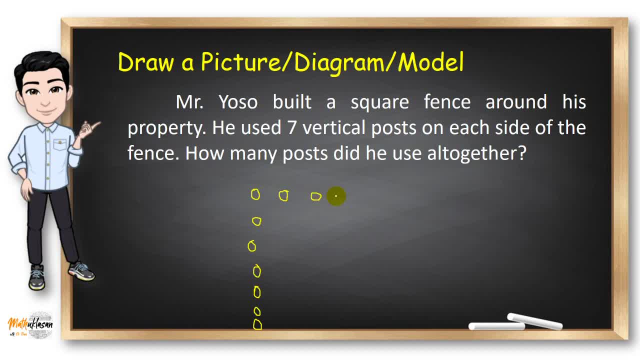 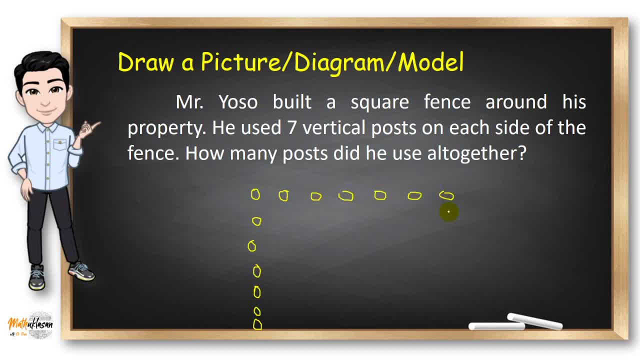 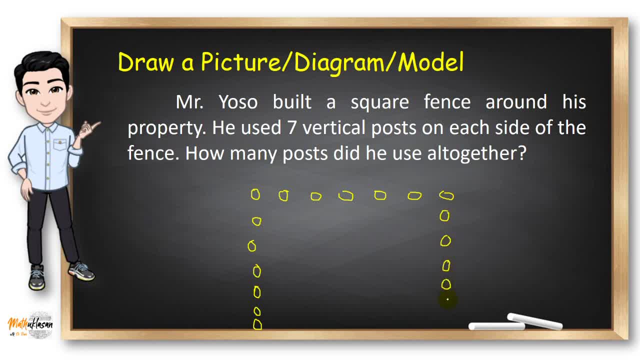 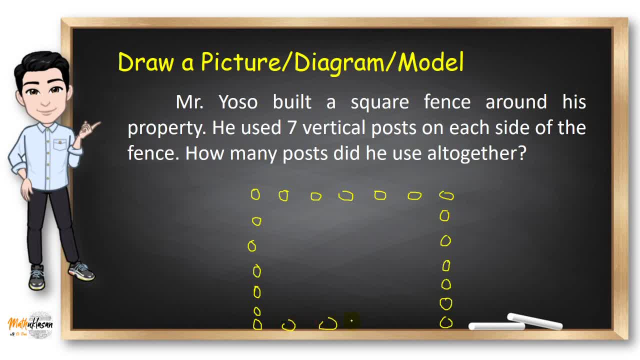 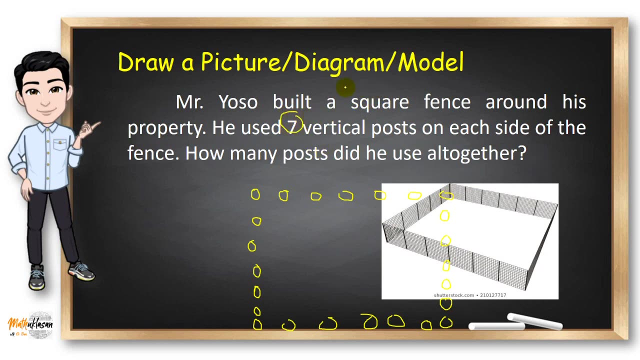 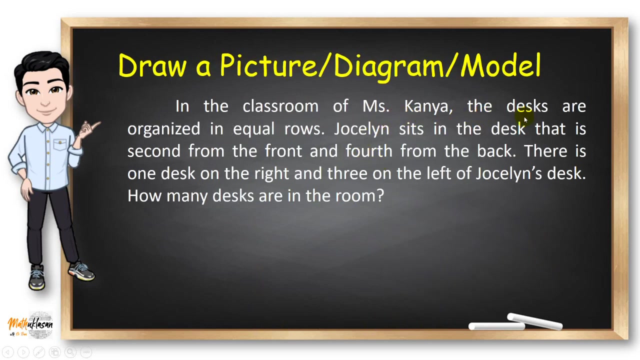 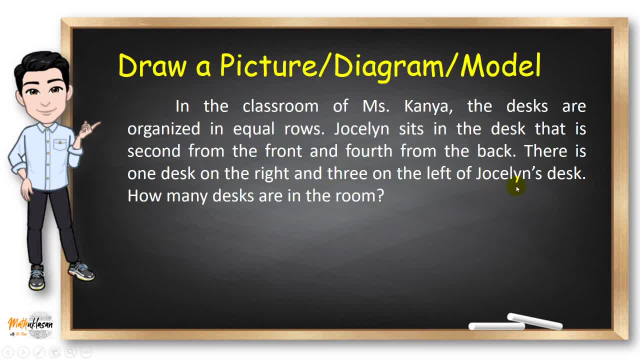 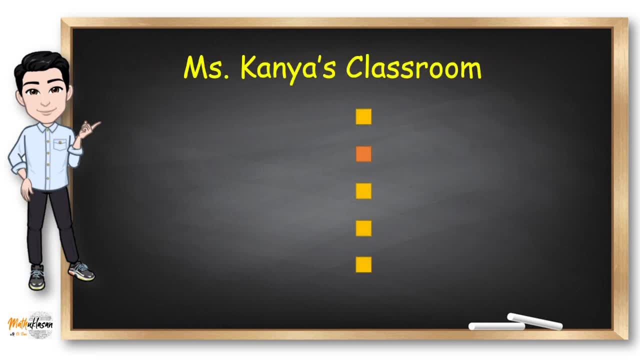 There is one desk on the right and three on the left of Jocelyn's desk. How many desks are in the room? So we could start by drawing the place of Jocelyn. So Jocelyn is second from the front, So there is one desk in front of her. So, since she is fourth from the back, 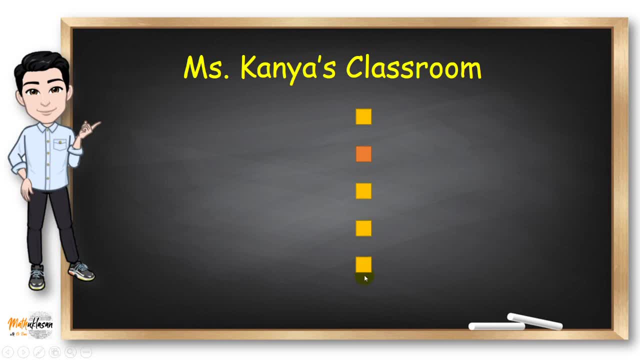 there are three other desks behind her or behind her. There is one desk on her right and three desks on her left. So therefore we have 25 students in the classroom, because all we need to do is to fill out the remaining. Since we have equal number of desks for each side, then we have 25 students or desks in the. 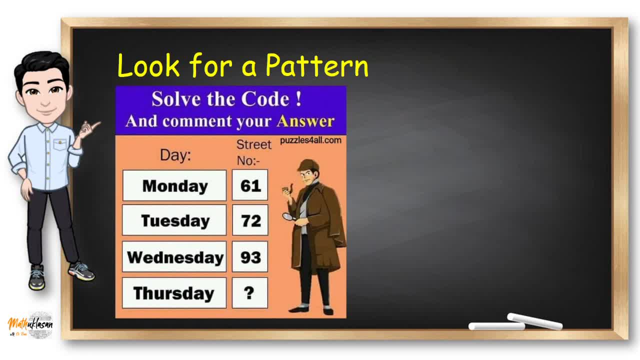 classroom. Math. patterns are sequences that repeat based on a rule, and a rule is a set way to calculate or solve a problem. By identifying the pattern in a problem, we'll be able to predict the answer In this problem. the days of the week are given up to Thursday and we need to 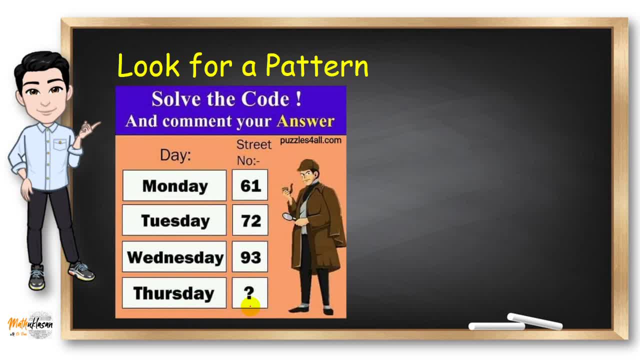 calculate the number of streets, that corresponds to Thursday. So here we can see right away the pattern: 1,, 2, 3 for the units digits. So this could be 4.. But how do we find the next numbers or digits on the left side of 4?? Notice that 7 was derived by adding 6 and 1.. 6 plus 1 is 7.. Therefore, 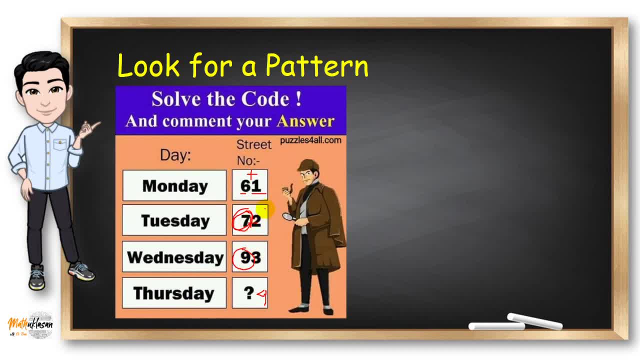 this 9 was derived by adding 7 and 2.. So therefore, to get the next digits on the left side of 4, we just need to add 9 and 3.. 9 plus 3 here is 12.. So the next number or the street we are looking. 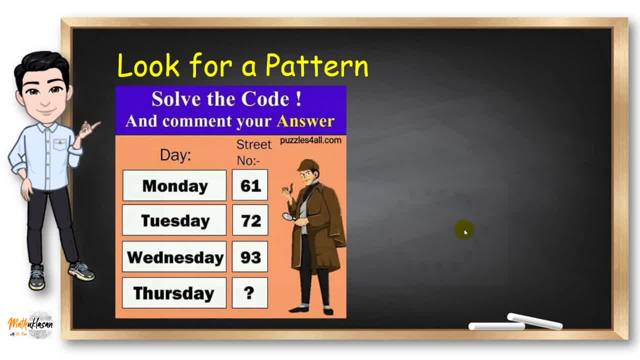 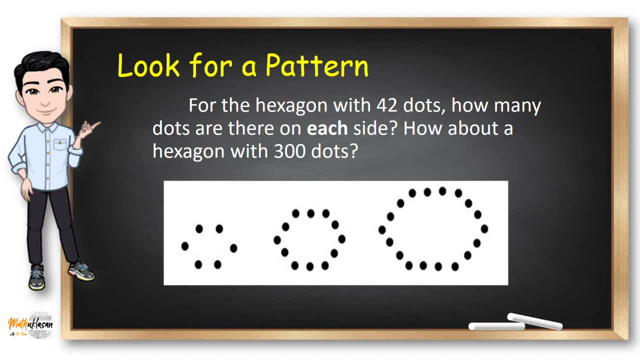 for is 124.. Sometimes we need to form different equations and mathematical expressions to solve a particular problem. For this example, we have a hexagon with particular number of dots with each side. For the hexagon with 42 dots, how many dots are there on each side? And how about the hexagon with 300 dots? 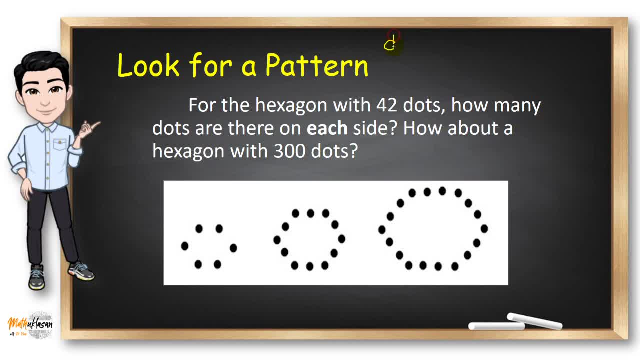 This time I'm going to represent D as the total number of dots in the hexagon and S for the number of dots in each side. So in the first figure notice that we have 6 dots. In the second figure we have 6сяч dots. For each dot we have 4.. And for each side we have a total of. 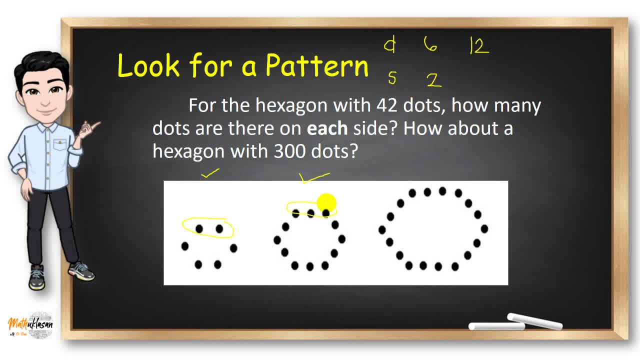 32.2 dots. For the second figure, we have a total of How many dots? We have 12 dots, andthat are 3 dots for each. In the third figure, notice that we have 18 dots, and that are four dots for each side. 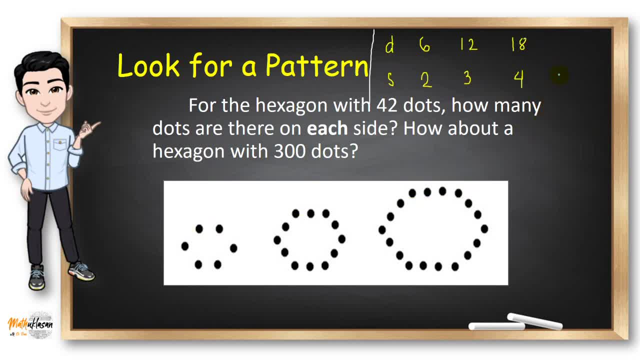 ック. I'm looking for the next answer for the total number of dots. if I have five dots on each side of the hexagon, So notice that 6,, 12, and 18 are all multiples of 6, and you can actually get 12 by multiplying 6 to 2.. So all we need. 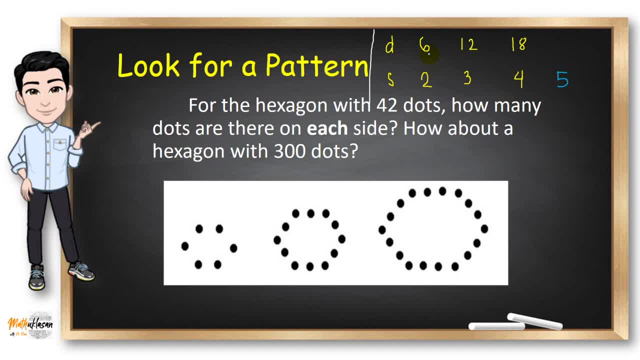 to do is to multiply what? Yes, we just need to multiply 6 to 4 to get 24, and to get 12, we need to multiply 2 to 6, and to get 18, we need to multiply 3.. So what I'm? 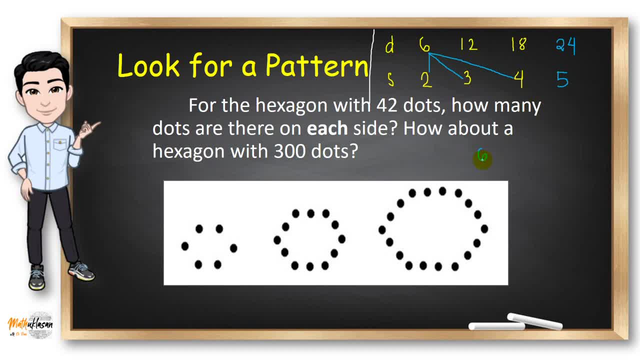 doing is multiplying 6, 2s minus 1, because let's say I'm looking for six, I need to use five instead. so six times five is 30 for you to get the next answer: total number of dots. So the formula or the mathematical equation for this is D. 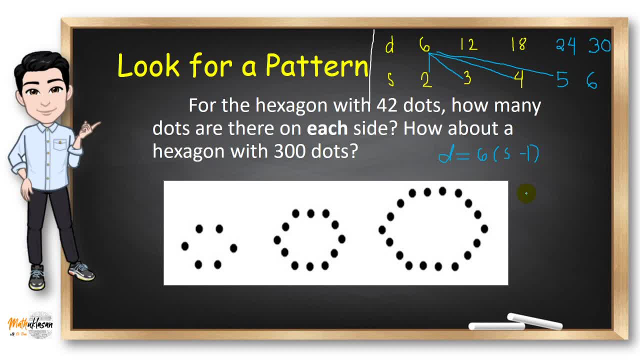 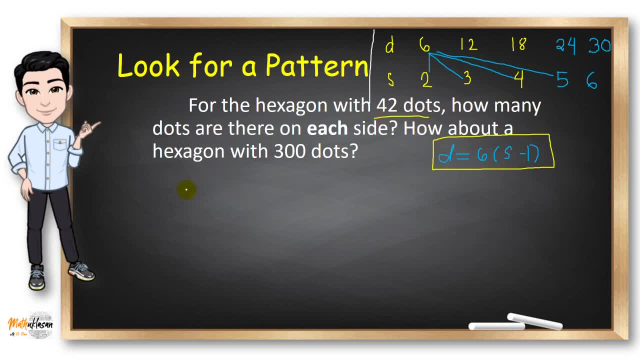 equals 6 times S minus 1.. And now we can use this formula to solve the problem. So if I have 42 dots, D is equal to 42. So all we need to do now is to solve for the value of S, to find the number of each side in a hexagon with 42 dots, By using your 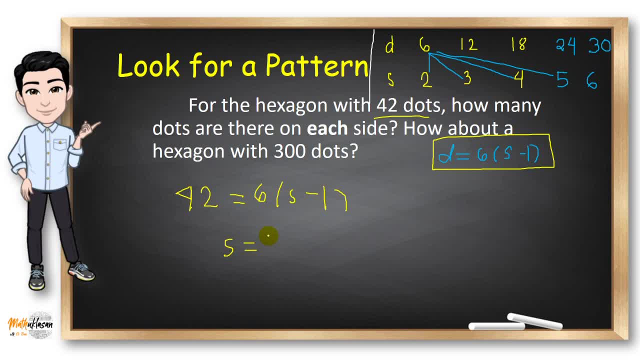 skills in algebra. S is just equal to what? Yes, it's just equal to 8.. Oops, forgot this one. Okay, So for a hexagon with 300 dots, all you need to do is to substitute 300 to D. 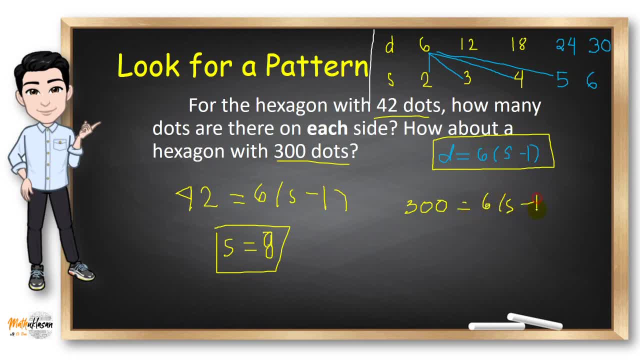 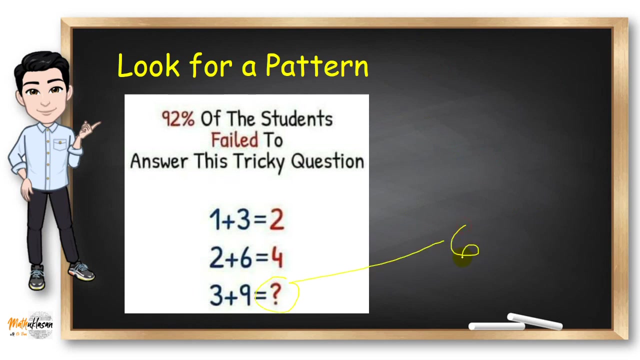 And then, using the same formula And by using your algebra skills and solving this equation for S, the answer is 51.. How about you try these examples? I'm going to tell you the answer. The answer here is 6.. But why In this problem? 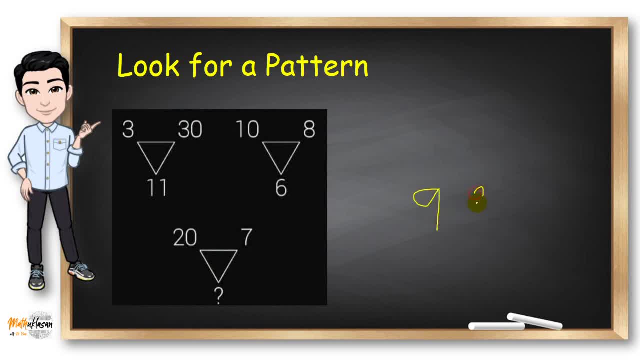 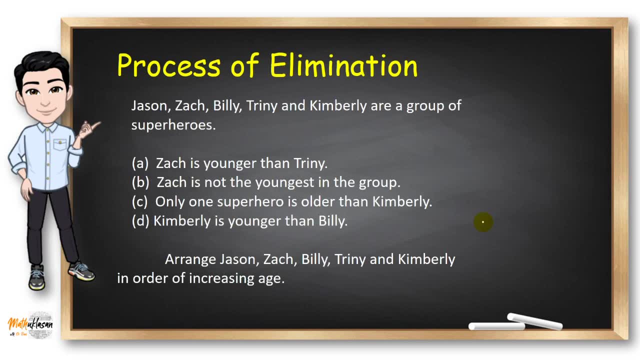 the answer is 9.. Again, why? Eliminating some of the possibilities is also one of the ways to solve a problem. So here, Jason, Zach, Billy, Trini and Kimberly are a group of superheroes, and we need to arrange the ages of these superheroes in increasing order. 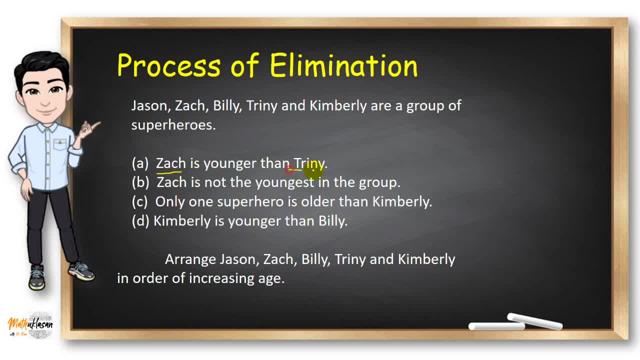 Our first clue suggests that Zach is younger than Trini, So if this is an example, then is Trini. Zach should be below Trini. Zach is not the youngest in the group, So there is always a younger superhero to Zach. In the third clue, only one superhero is older than Kimberly. 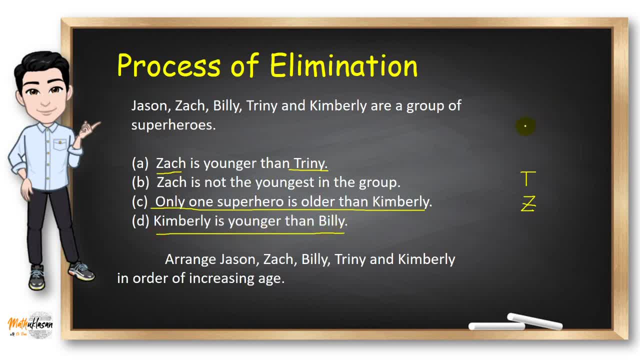 So if Kimberly is younger than Billy, then it must be Billy and then Kimberly. Now remember that Zach is not the youngest in the group, So there is another one person who is younger than him. Who is he? Yes, it's Jason. So the youngest is Jason, followed by Zach. 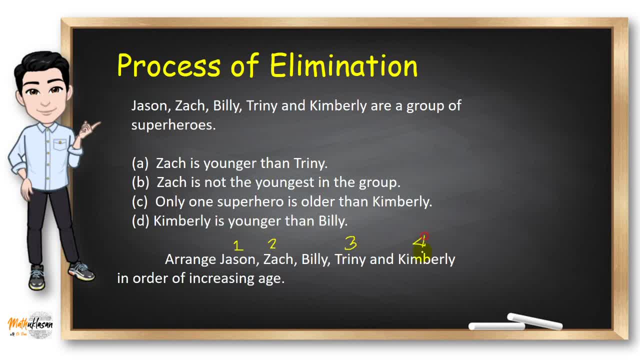 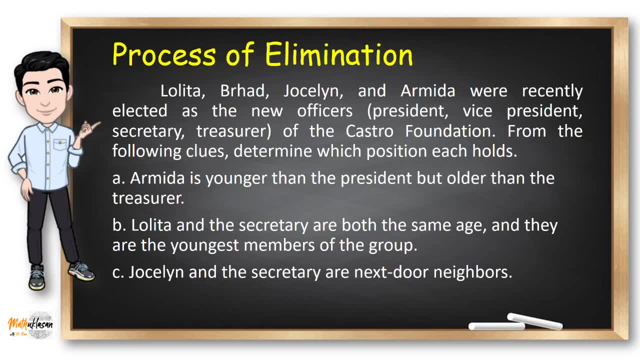 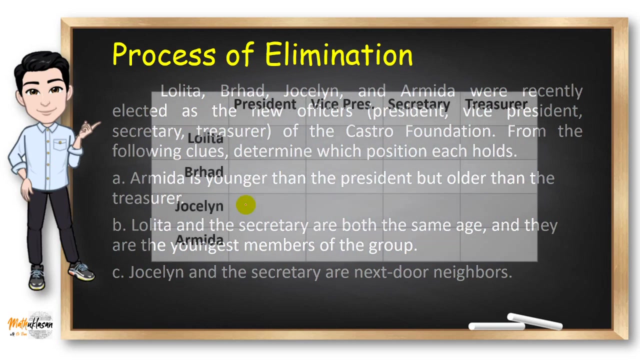 Trini, Kimberly and Billy as the oldest one. Let's try another example. Lolita, Brihad, Jocelyn and Armida were recently elected as the new officers of the Castro Foundation. From the following clues: determine which position each holds For the elimination: 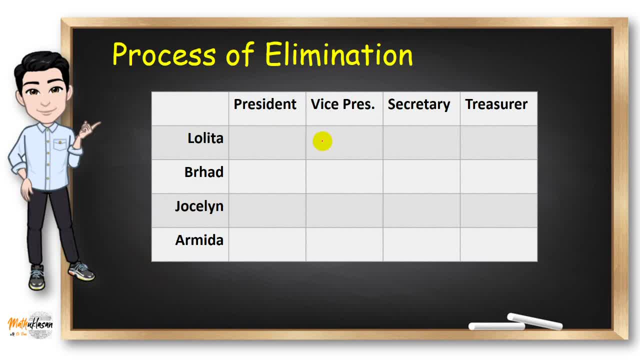 process. we can use this table containing the names and the positions. The first clue says that Armida is younger than the president, but older than the treasurer, So she can't be the president. The second clue tells us that Lolita and the secretary are both the same age, So Lolita can't. 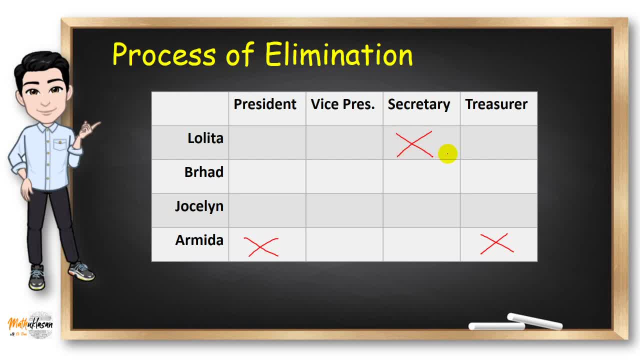 be the secretary And they are the youngest members of the group. So Armida is also not the secretary, because Armida is older and not the youngest. For the third clue, Jocelyn and the secretary are next door, So she can't be the secretary because she wants to have more buses, So Jocelyn is the secretary. 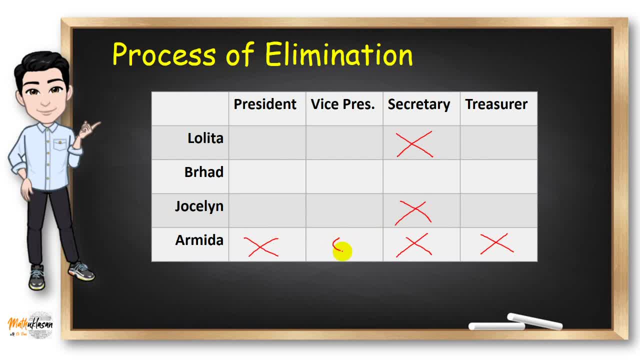 From this elimination, we can now say that Armida is the vice president because it's the only option for her, While Brihad is the secretary because this is the only available self for this column Now. so Brihad is not the president, the vice president and the treasurer, So, Jocelyn. 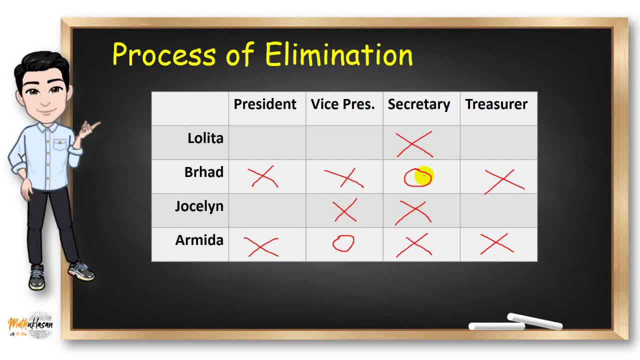 the vice president now, since Brihad, or the secretary, has the same age with the treasurer. so therefore Lolita is the treasurer because they're both the youngest in the group and the only available slot now for Jocelyn is president. so the president is Jocelyn, the vice president is Armida. the 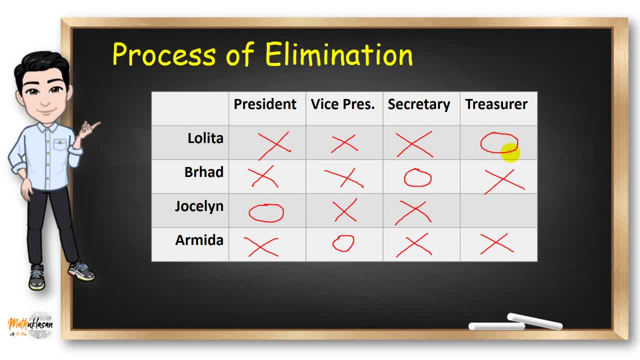 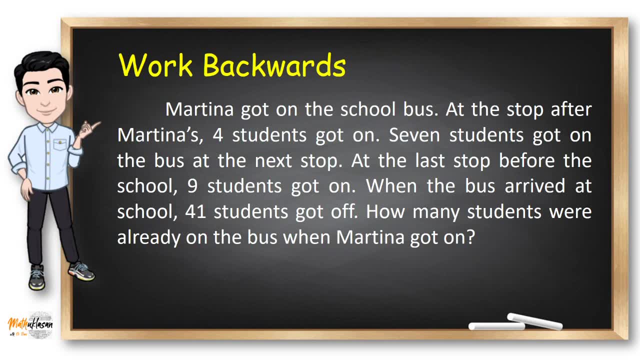 secretary is Brihad and the treasurer is Lolita. when a succession of events are involved, working backwards is one of the strategies that we could use in this example. Martina got on the school bus at the stop after Martinez for students got on. seven students got on the bus at the next up, at the last stop before the 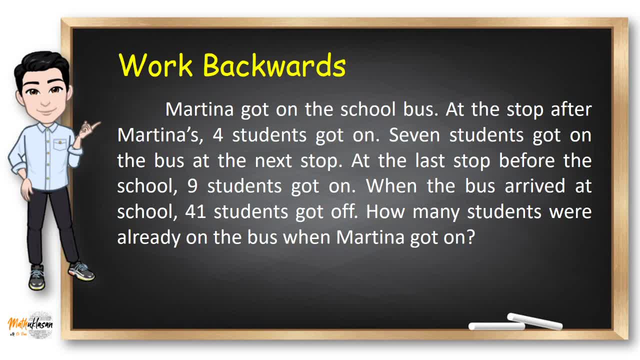 school, nine students got on. when the bus arrived at school, 41 students got off. How many students were already in the bus when Martina got on? Since 41 students got off the bus, the total number of students inside the bus is 41..